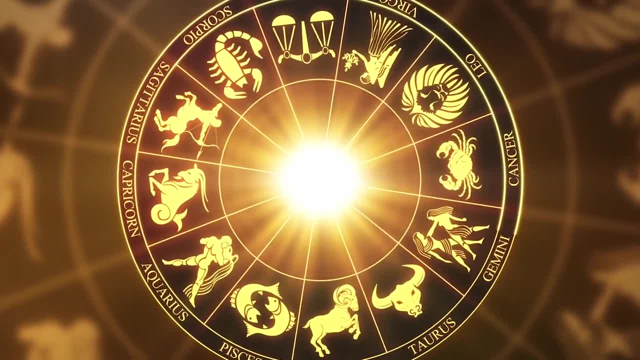 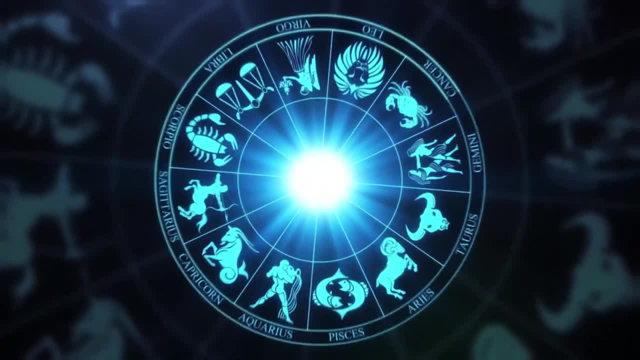 including one referencing the Greeks, which is what we'll be referring to here, and the Chinese Zodiac, for which they label a year after whatever animal is next in the Zodiac. But for the Greek one, what does it reference? what does it all mean? 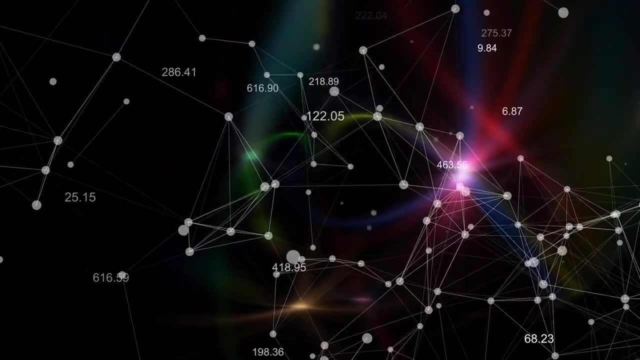 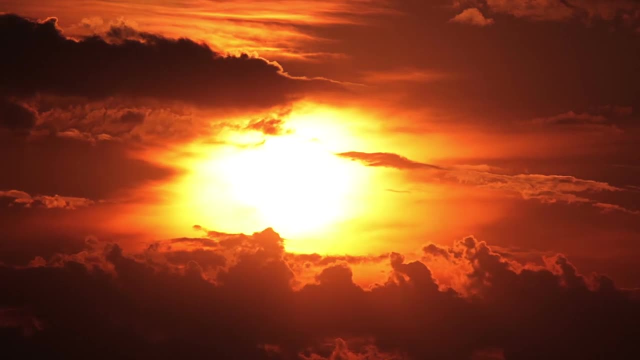 To keep it very basic, the Zodiac is a series of 12 constellations that are in ecliptic, or in the path of the sun, our sun. So thus these 12 are seen as special because the sun passes by them when it moves, Or at least that's how we perceive it here on Earth. 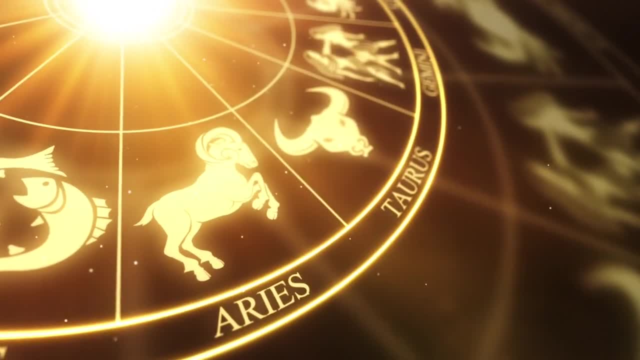 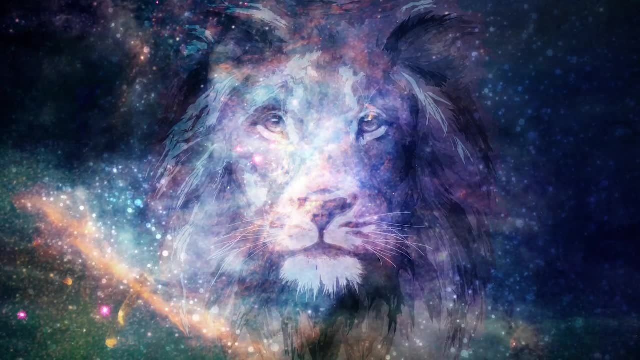 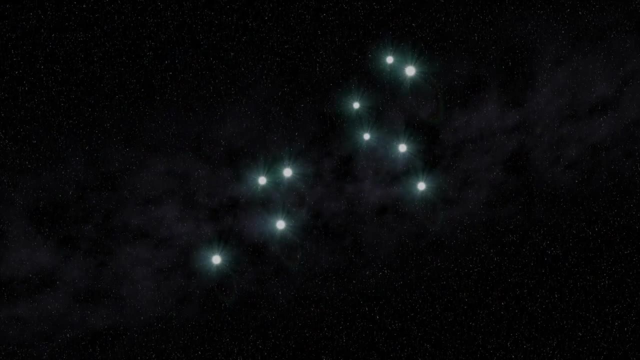 Now, as for where the word Zodiac comes from, that would be from the word zodiacos, which means circle of animals, which is poetic because all of the constellations, save for one, represents living animals in our world today, And because there are 12 constellations in the Zodiac. 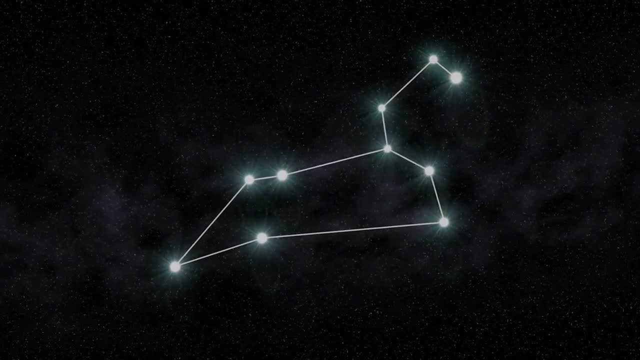 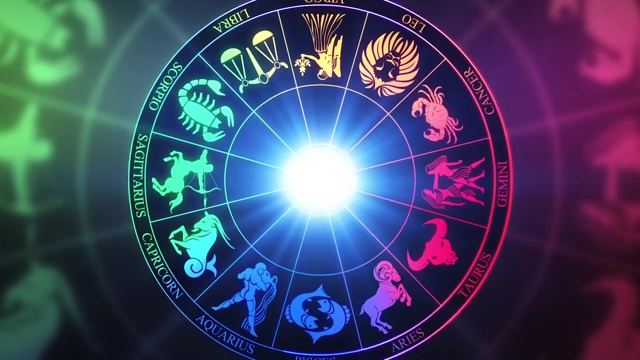 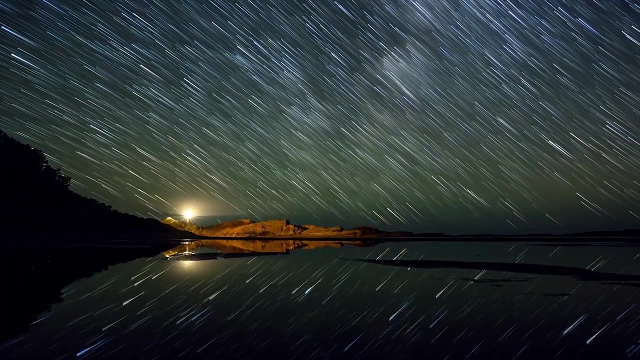 and 12 months of the year. we've assigned special dates to them, based on the position of the sun when it passes through them, and thus we get the signs, which eventually add two horoscopes, and that's another list entirely. So, knowing all of that, shall we get started on the significance and details of each constellation? 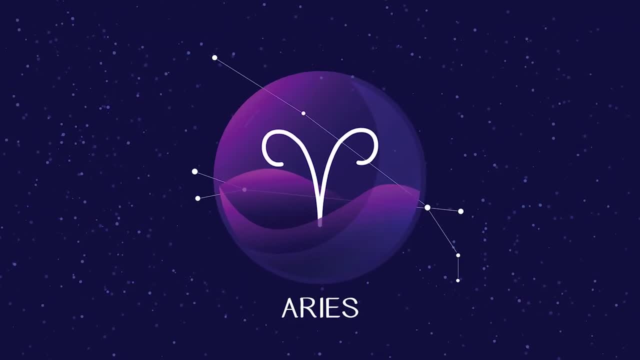 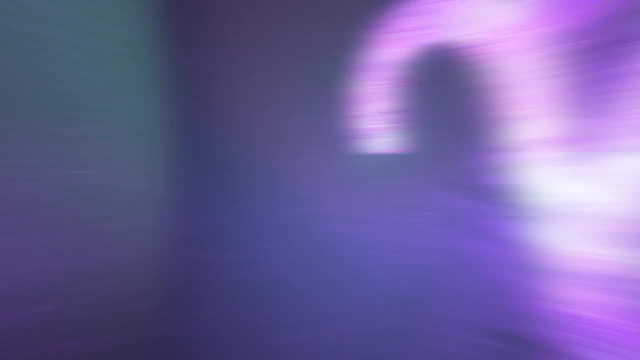 12. Aries, Not to be confused with the Greek god Ares, Ares is a ram and is passed by the sun between April 19th till May 13th. As for the stars that make it up, that would be Hamal, Sheraton, 41 Ari. 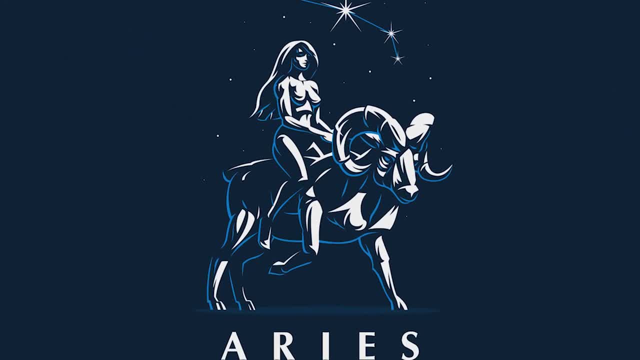 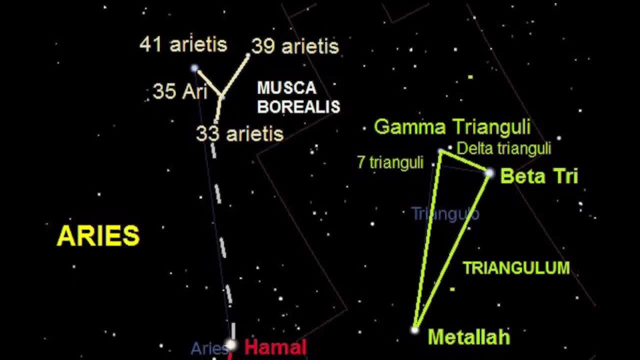 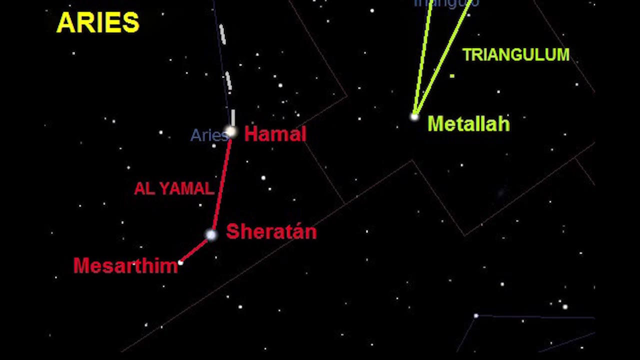 Botene, HD 20644,, E, Ari 35, and Y2 Ari- Yeah, that's a mouthful, isn't it? The constellation is quite a ways away, such as with its brightest star, Hamal, which is 66 light years away from where Earth is. 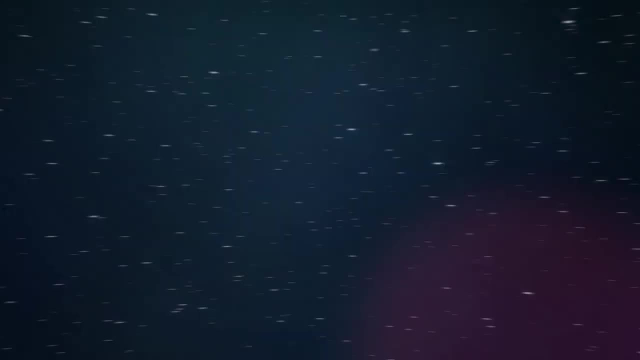 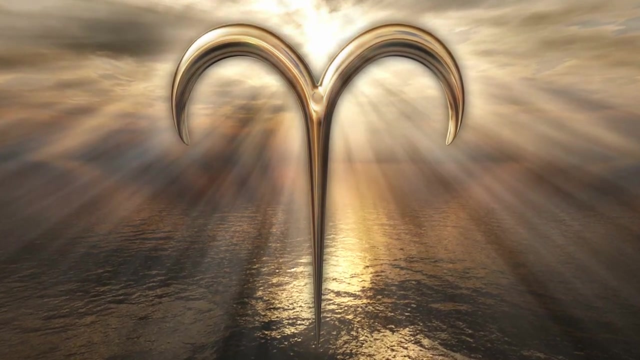 Yet that proves how bright it is, so we can see it from Earth itself. Aries the ram is depicted many different ways across many different mythologies, including ones in both Western Egyptian and the Greek. In terms of Greek mythology, the ram known as Aries was one with a golden fleece. 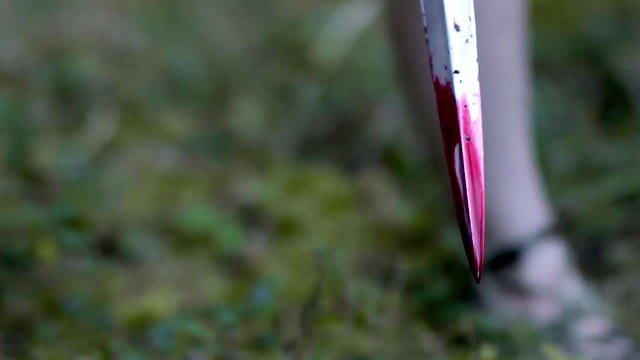 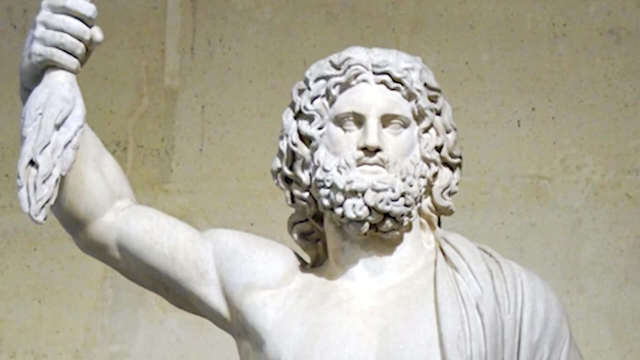 one that helped save the sun from being sacrificed by his father after a conspiracy had been hatched to kill them. The ram was later sacrificed to Zeus and the fleece was given to him as a tribute, who later gave it to others, who then hung it in a cave guarded by a dragon. 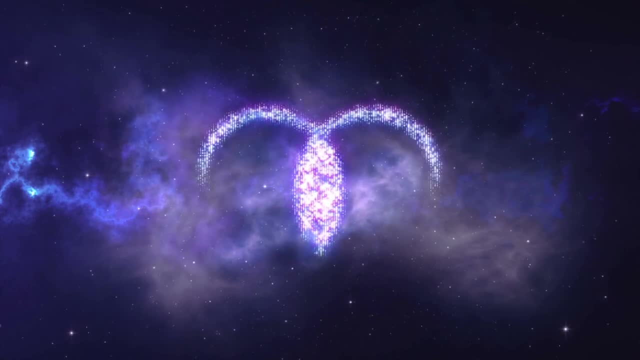 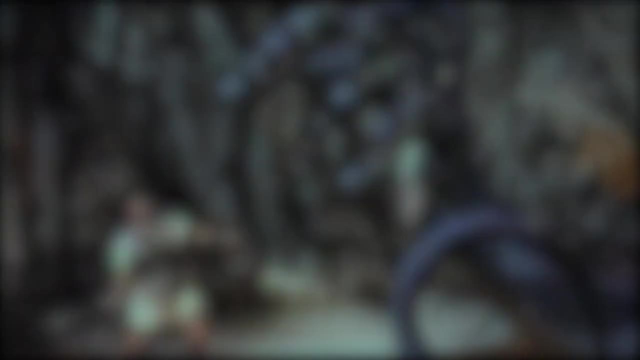 Also, though, for those who know their Greek tales, you'll know that the golden fleece was the goal reward of Jason and the Argonauts, and they were able to steal it successfully. 11. Taurus, 11. Taurus, 11. Taurus. 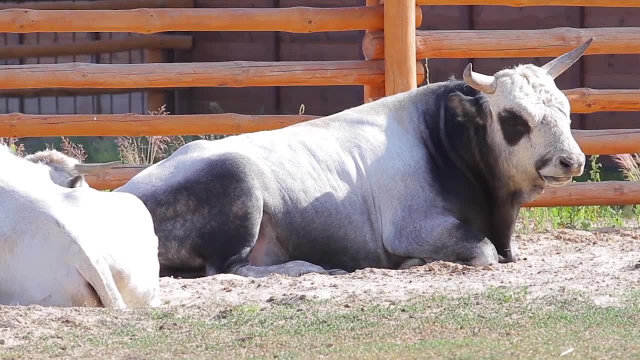 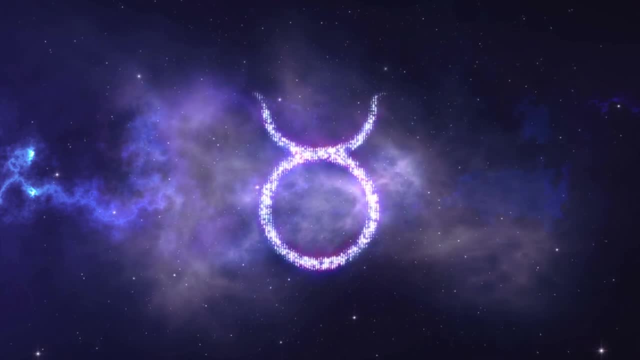 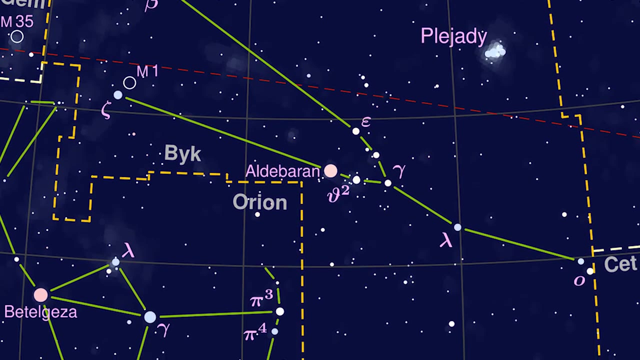 Anyone feeling rather bullish today, You know because, as a bull, Never mind. In terms of the path of this constellation, it is crossed by the sun between May 14th till June 19th. The stars that make it up include Aldabaran, Elnath, Alcyone. 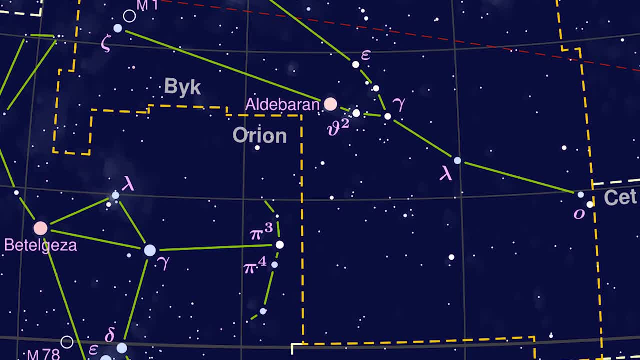 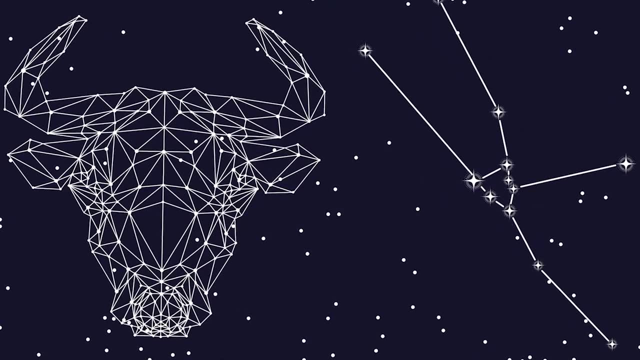 Zetao and O2tau2.. Try saying some of those names five times fast. Taurus is actually quite far away from Earth, almost 400 light years away, so don't expect to see it up close, Not unlike Aries. there are many different depictions of Taurus, the bull in both mythologies. 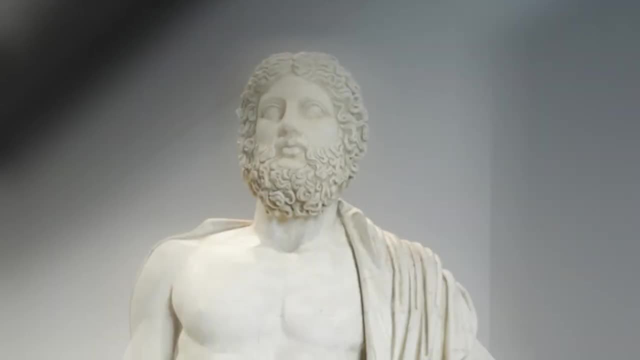 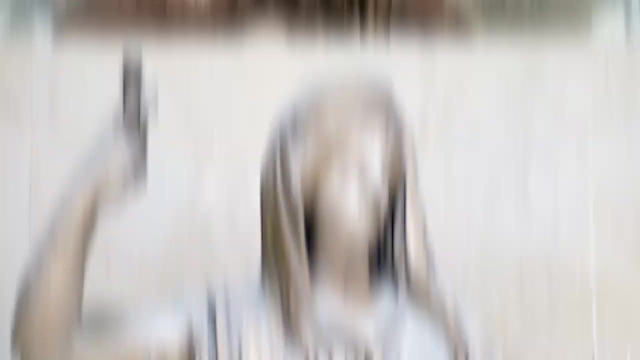 abroad and Greek mythology itself. For example, there are many references to the bull being Zeus, who was known to shapeshift all the time to be close to his many mistresses. One story even states that he turned one of these mistresses to a bull to hide her from Hera, who was known 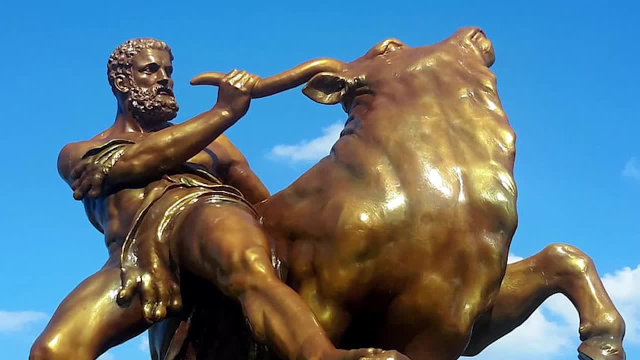 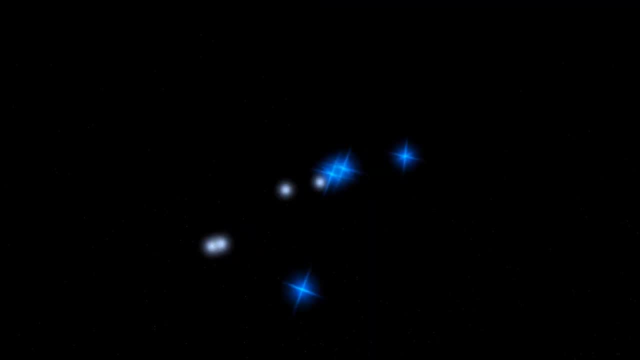 for jealousy and lashing out at said mistress. Others, though, believe that it could be a reference to Cretan bull, that Herakles was the one who was known to shape-shift all the time That Herakles had to deal with in one of his many labours. Either way, the bull became not. 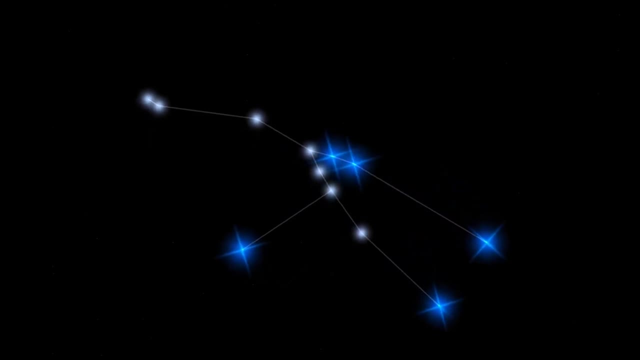 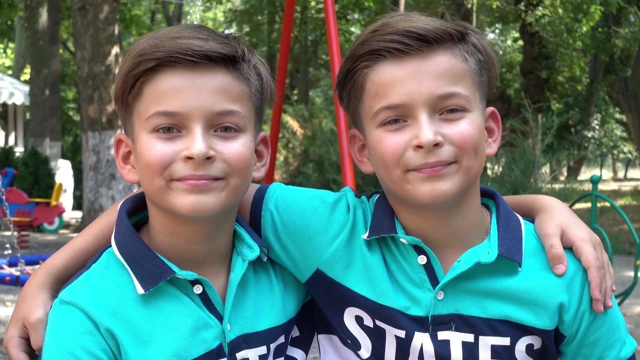 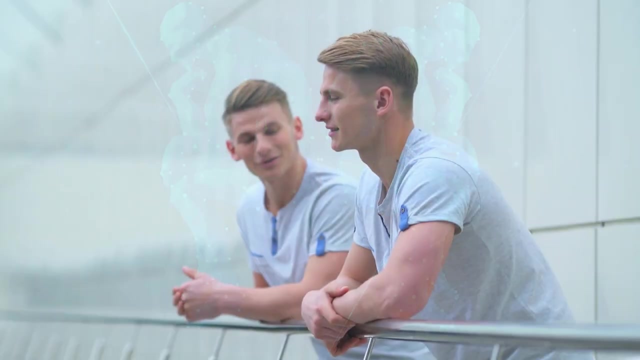 just a constellation, but a figure of many different mythologies, including ones worshipped to this day. 10. Gemini- Ok, how many twins in the house? No, really, I'm curious, And it's poetic because Gemini is a term that is used in pop culture and culture the world over to talk about the twins of the world. 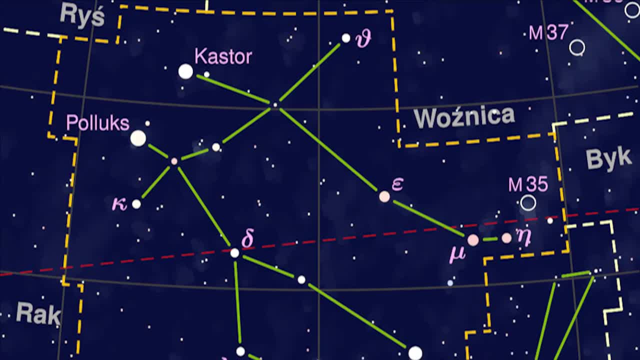 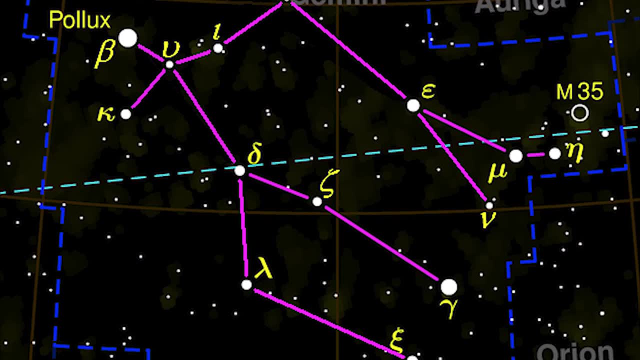 including a recent movie, Gemini Man. As for the stars, there are 85 stars that technically make up the constellation, but the main ones are Pollux, Alhena, Castor A, Taget Posterior and Castor B, to name a few. Again, there are 85 of them. 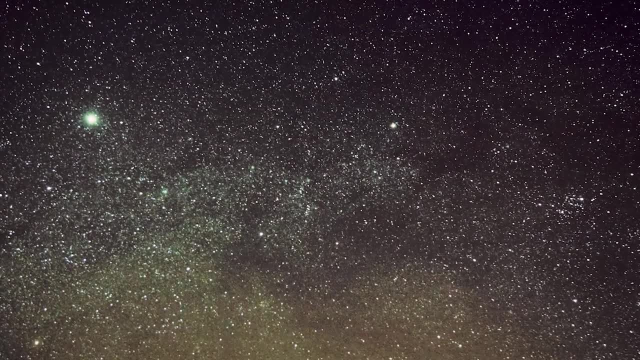 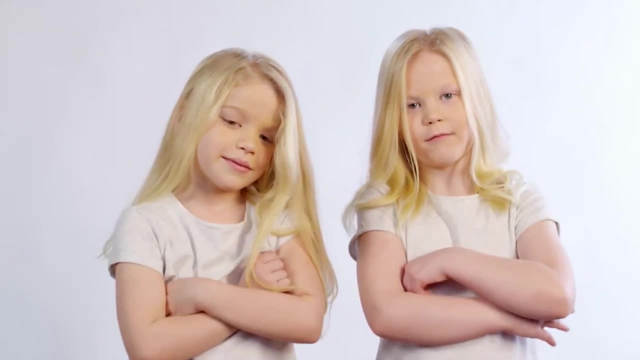 and that's just the ones we can see. In terms of distance. the closest star of the constellation, Taget Posterior, is 230 light-years from Earth. Going to the Greek mythology text for the origin of the twins, well, let's just say it's a bit messy. You see, while they were twins, each boy 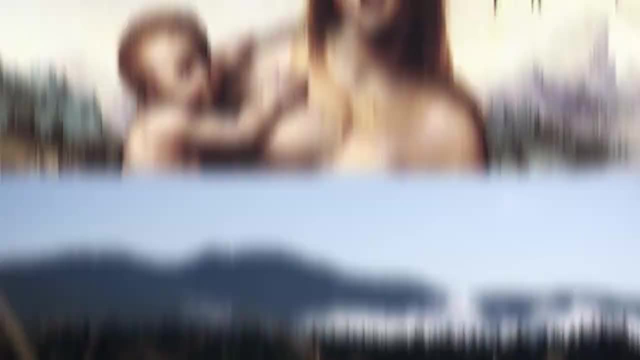 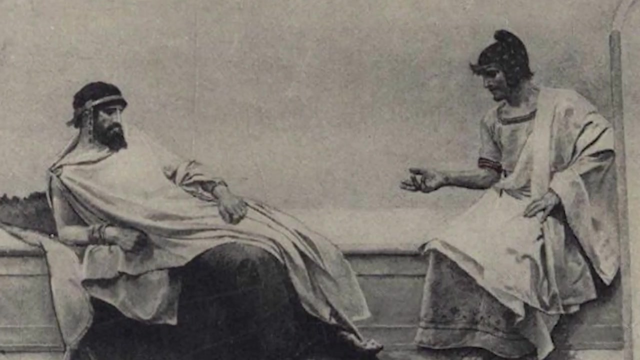 Pollux and Castor had a different father. I'm not saying a word. Anyway, their mother was Leta, but Zeus was the father of one and the Spartan king Tyndareus. again, I'm not going there. 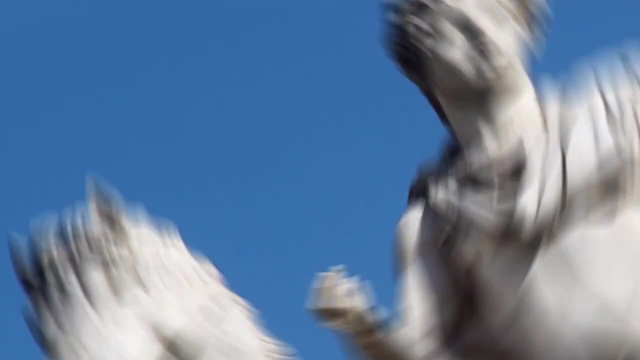 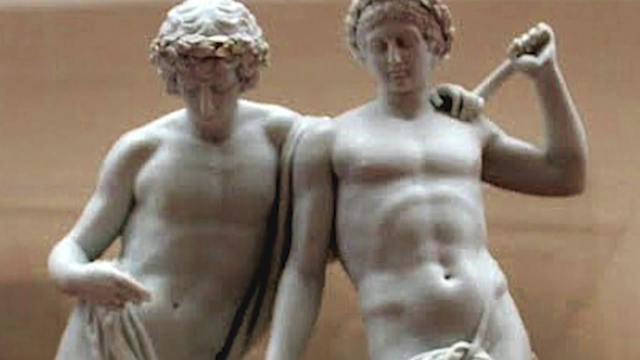 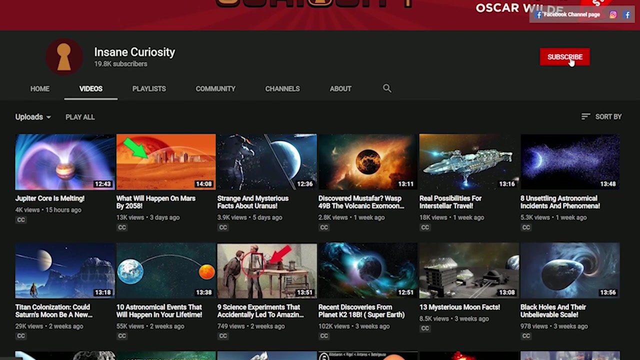 The problem here was that, because Pollux was a demigod, that made him immortal, but Castor was mortal thanks to his human father. Thus, when Castor died, Pollux implored Zeus to let him live forever, So the two were put together in the sky. Before we break down more of the constellations, 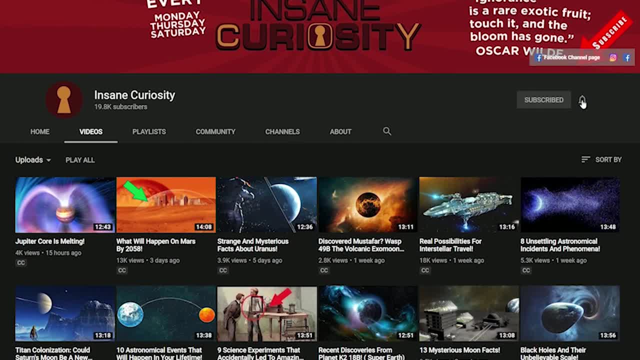 in the zodiac. before we break down the constellations in the zodiac. before we break down more of the constellations in the zodiac. before we break down more of the constellations in the zodiac, be sure to like the video and subscribe to the channel. That way you don't miss all of our weekly 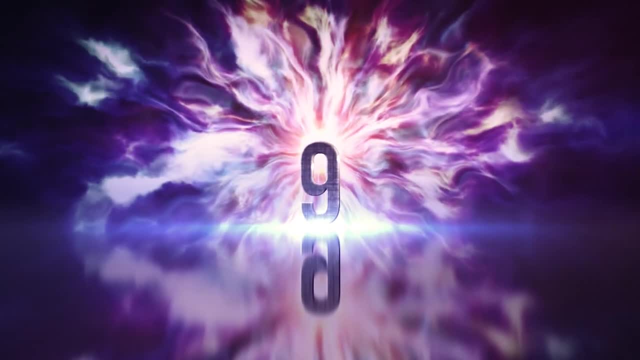 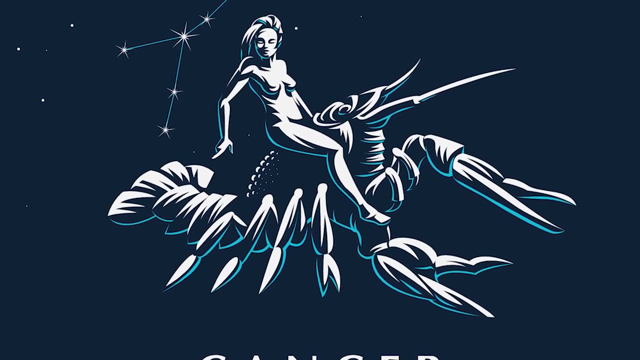 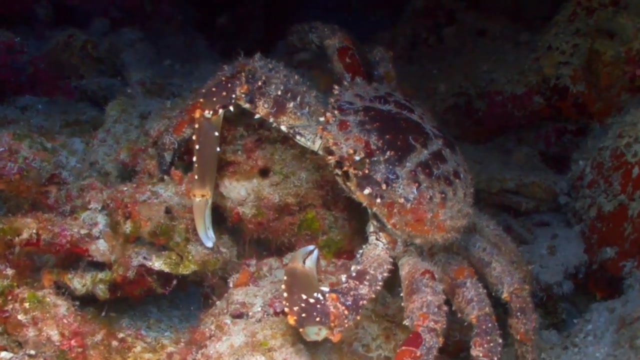 videos 9. Cancer- No, I'm not going to ask the obvious question. That would be insensitive. However, I will say that Cancer is, without a doubt, one of the most known constellations, if for no other reason than it's a crab and people just connect to it for some reason. It appears with the sun from July. 20th to August 9th. Some of the stars in the constellation include Al-Tarif, Acellus Australis, Acubans, Acellus Borealis and more. It's also about 131 light years from. Earth in regards to its closest star. Remember when I said people just related to Cancer? Well, here's why Its story is very sympathetic. So you remember the beast known as Hydra, right? Well, after Heracles slew the monster, a crab named Cancer came around and bit Heracles on the foot. 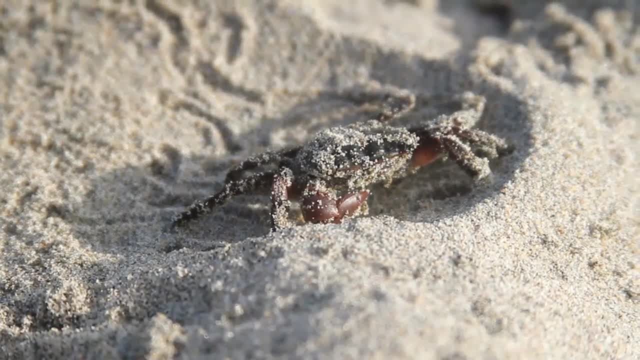 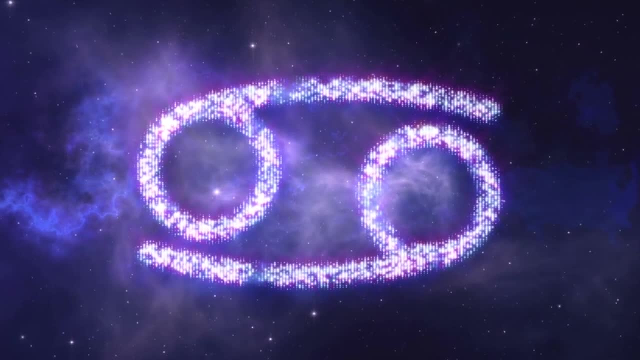 Not taking kindly to that. Heracles killed the crab. End of story, right? Not so much Hera, if you recall I said, was the jealous type, decided to spite Heracles by taking the crab and putting him in the sky for all to see. 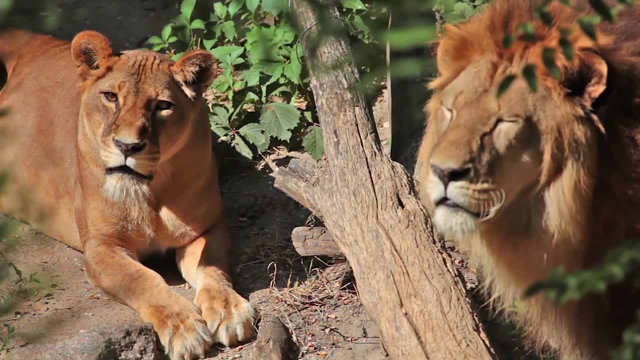 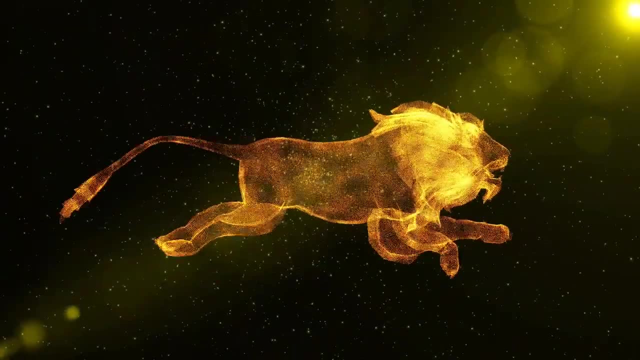 8. Leo. Lions across the world are part of many mythologies, including being the symbols of strength, power, courage and more. So it would have honestly been odd if there wasn't a lion constellation in the sky. I'm just saying, Anyway, the constellation known as Leo. 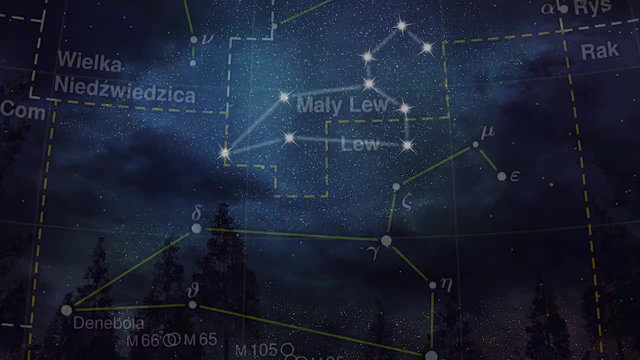 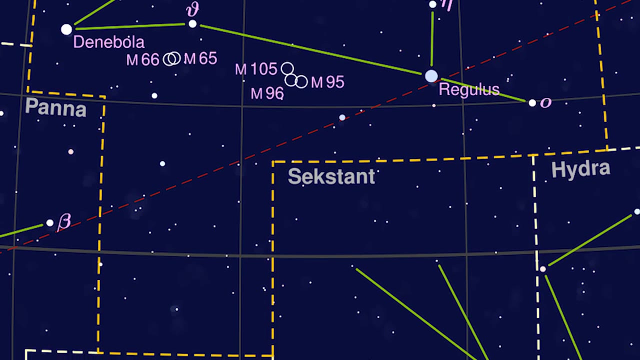 passes by the sun from August 10th till September 16th and is made up of many stars, including Regulus, Denebola, Zosma, Algeba and Ros Alast, Australis, Oh, and it's 247 light years from Earth. 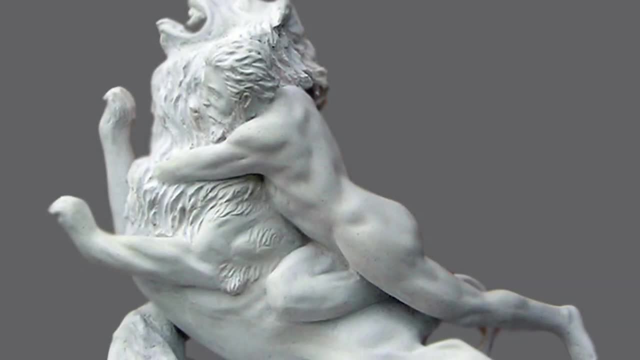 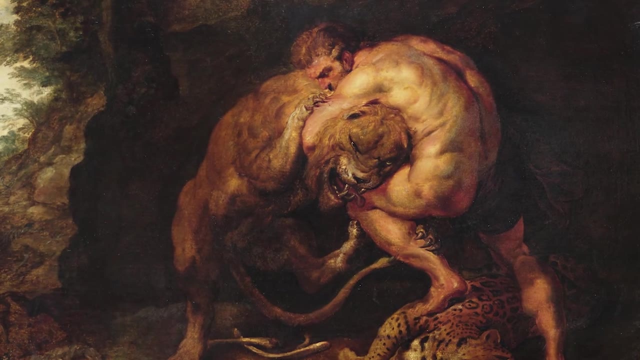 to its closest star, Leo. the lion has a prominent place in Greek mythology as it was the first of 12 labours of Heracles. Specifically, it was the Nemean lion that Heracles successfully killed. Oh, and by killed, I mean that Heracles had to be killed to be able to survive. Heracles had to be. 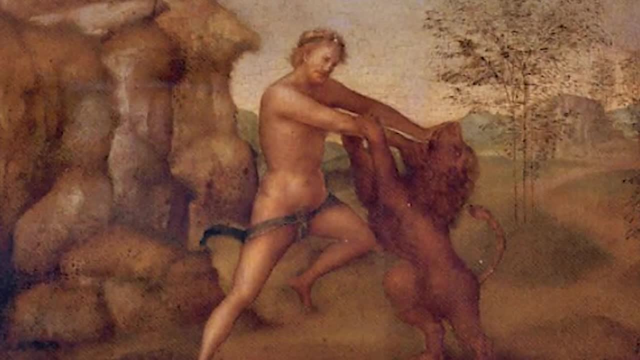 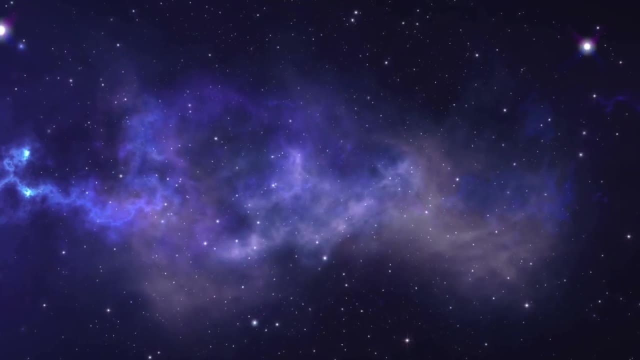 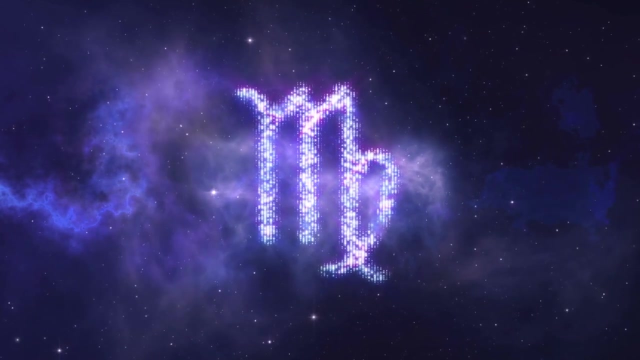 beaten with its bare hands by bending it so far backwards that he broke the lion's back. That's hardcore. 7. Virgo. Virgo is revered as one of the constellations we can most easily observe in our skies, and it passes by the sun from September 16th till October 30th. Some of its stars include Spica. Vindimitrix, Eze, Auva, Zavachava and more. It's also 260 light years away from Earth. Of all of the constellations, Virgo is one that is the most plentiful in terms of interpretations. 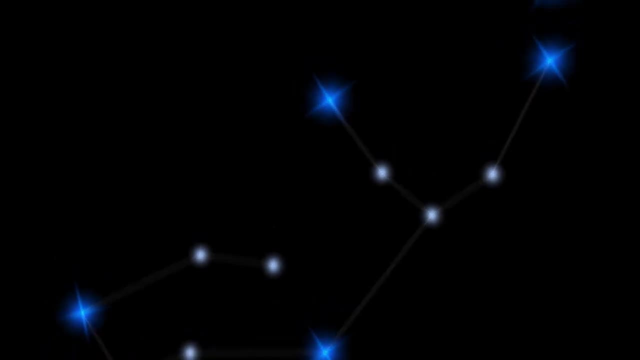 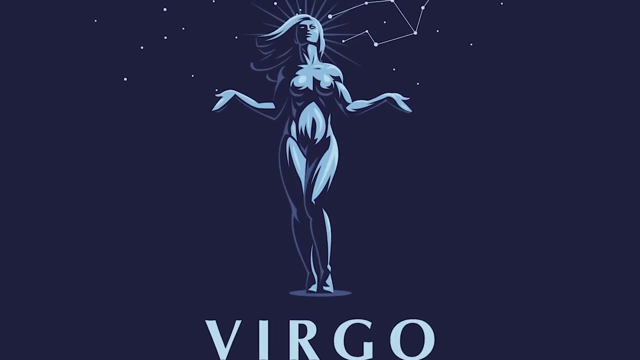 Even the Greek mythology texts debate what it's supposed to represent, including it being the goddess Demeter, who is the goddess of agriculture. Other interpretations have it as other goddesses, including the one of virgins or justice itself. Some even think it's. 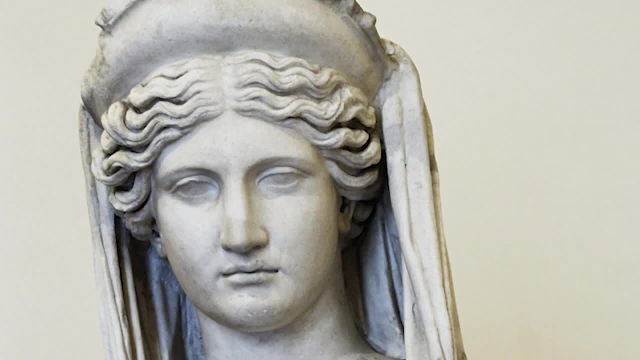 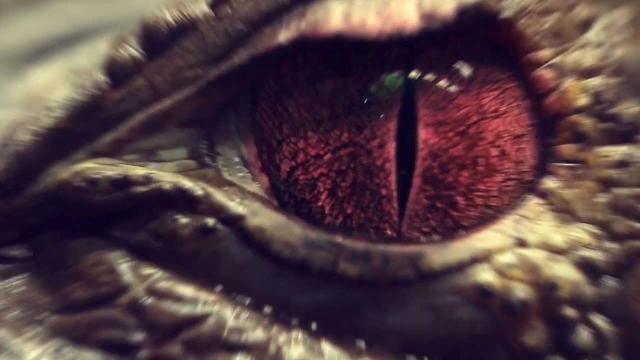 supposed to be a legendary Greek monster. I'll take the agriculture goddess. I'm just saying I mean, would you rather picture a horrifying monster in the sky, or would you rather picture a sky above looking down on you, or a goddess that you can pray to to have a better harvest? 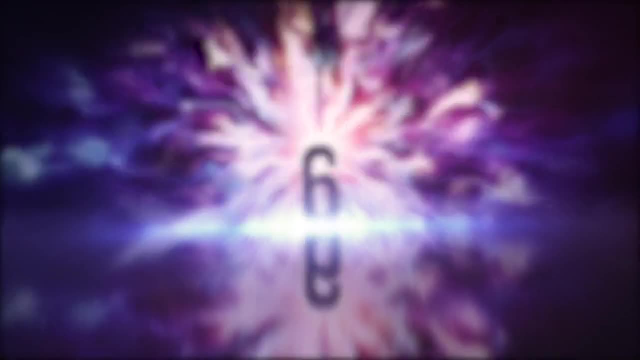 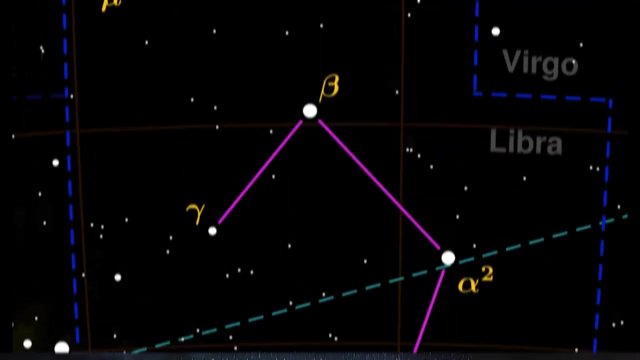 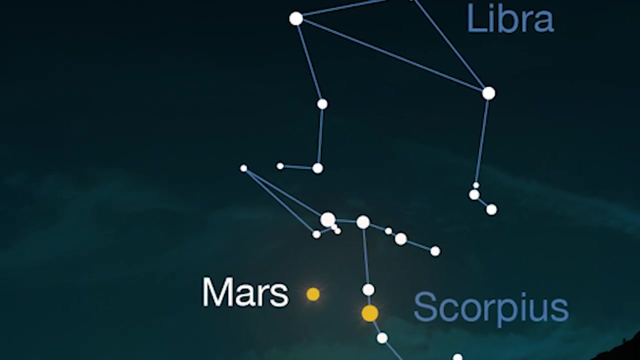 That's what I thought. 6. Libra. Libra is a constellation that is passed by the sun from October 31st until November 22nd. Its main stars include Zubinashimali, Ilanubi, Sigma, Librae and more, Though it's closer than many. 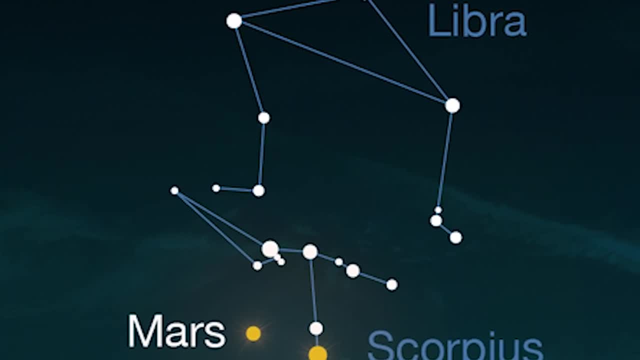 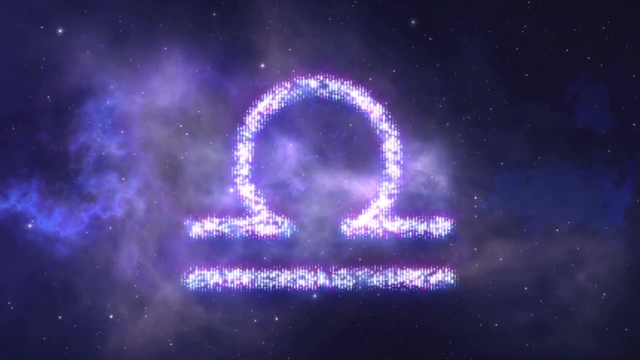 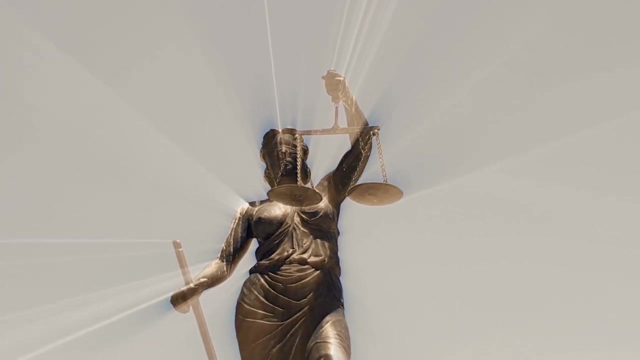 other constellations at only 185 light years from Earth. Libra is technically a person, but over the years the interpretation of the constellation changes from a person to scorpion's claws, to the scales of justice or just a regular weighing scale. The reasons are based on the cultures. 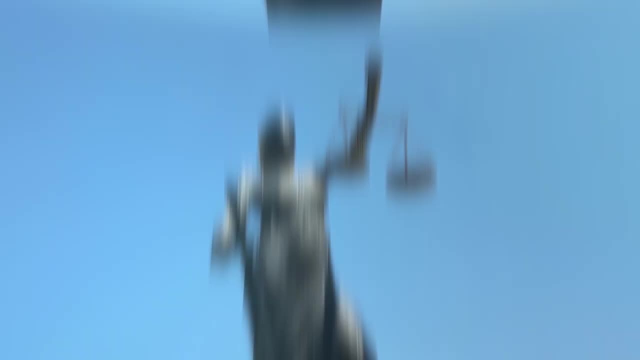 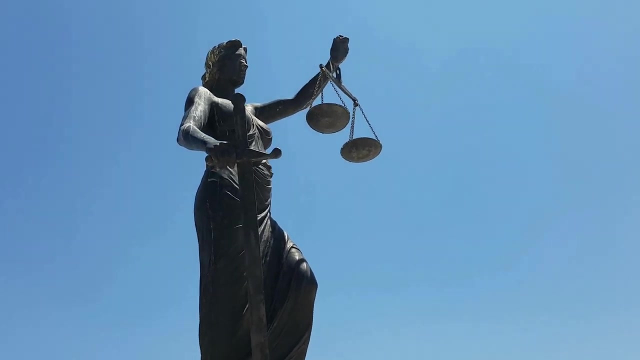 themselves. but one interesting thing to note is that when the sun passes by the constellation, the balance of the days and the nights are equal. thus the scales are even. Take of that what you will. of course There are other interpretations you can check out if you feel the need for a better. visual 7.. Libra is a constellation that is passed by the sun from October 31st until November 22nd. Its main stars include Zubinashimali, Ilanubi, Sigma, Librae and more, Though it's closer than many other. constellations at only 185 light years from Earth, Though it's closer than many other Orlando events. It's also known as Scorpio by theaming. At one time, Scorpio and Libra were thought to be part of the same constellation. That's why Libra was first known as the Scorpion's Claws. 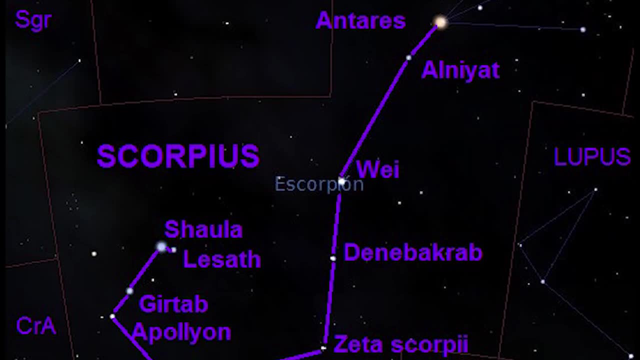 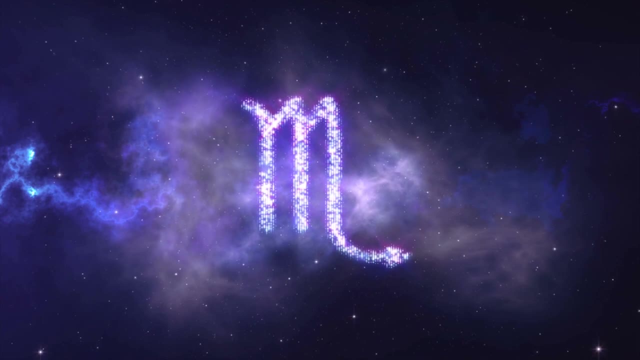 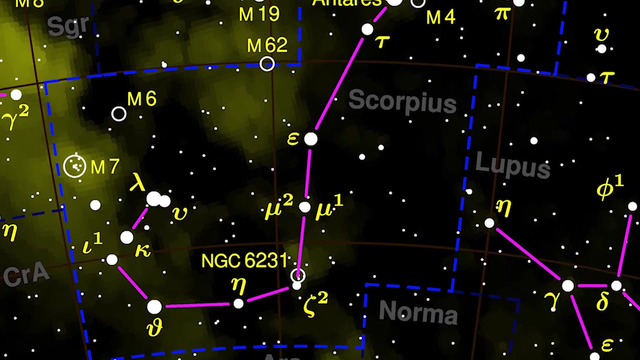 which became the scales. Eventually they were separated and Scorpio is now its own thing. As its own thing, the constellation gets passed by the sun on November 23rd till November 29th, and some of its main stars include Antares, Shaula, Sargas, De Shuba and more. But dear gosh is this one far away. it's 5500 light years from Earth, which should be a signal to you in regards to just how bright and powerful this constellation is Now. as noted, there was one time when Scorpio and Libra were one constellation that were. 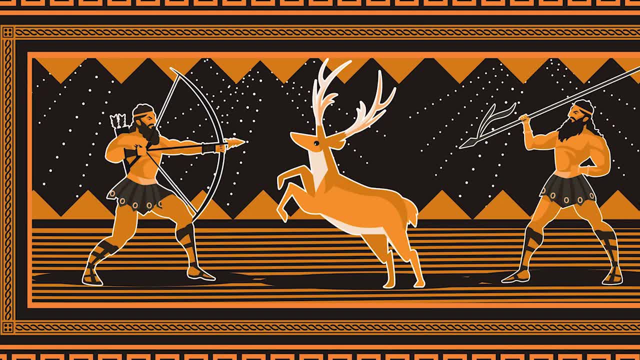 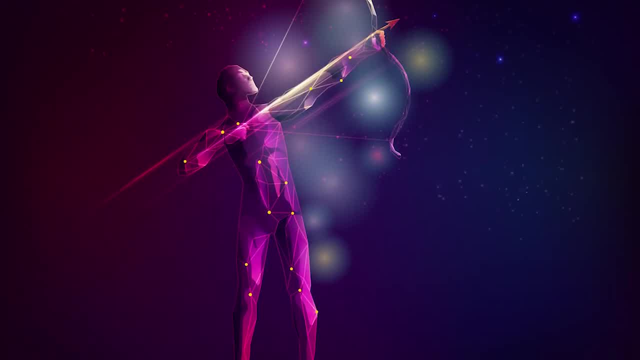 a reference to a scale of justice, but when referring to Scorpio itself, that would tie it to the legends of Orion the Hunter. Once upon a time, Orion stated that it could kill any living creature, so the goddess Gaia sent a scorpion after him with impenetrable armor. You know she cheated. He did get away from the scorpion, but the goddess Artemis unwillingly struck him down. Another take says that it was Artemis and her mother that sent the scorpion and the scorpion killed Orion. Zeus saw the battle between the two and decided to raise both of them to the sky to honor. 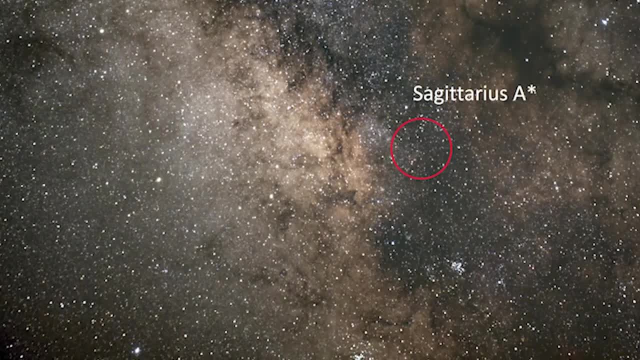 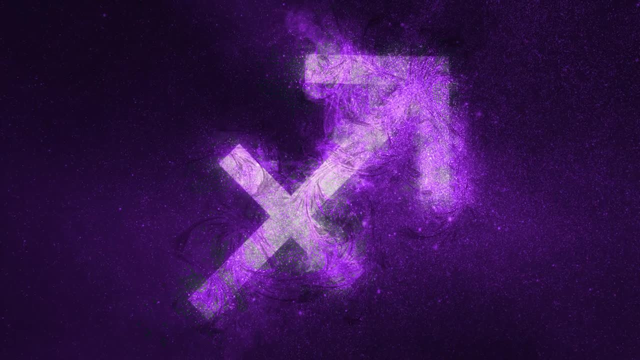 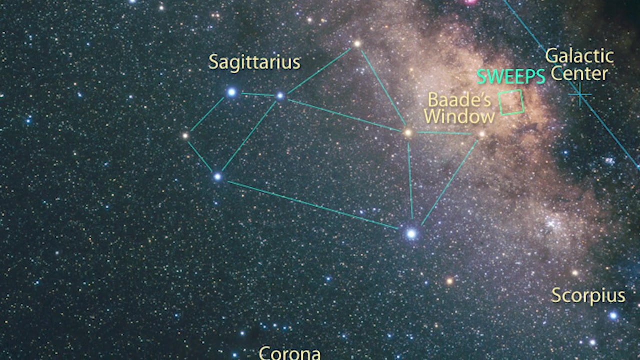 them. 4. Sagittarius: Sagittarius is a very curious constellation that is up in the sky Only because of the form it takes. It's passed by the sun from December 18th till January 18th. Its main stars include: Caus Australis, Nunci Acela, Caus Medeus, Caus Borealis. It's also another constellation that is a long way from Earth, over 5,000 light years away. As for what a Sagittarius is, you need only look at what it is in most of its depictions, meaning that it's a centaur, a creature that is half man and half horse, who have a rich 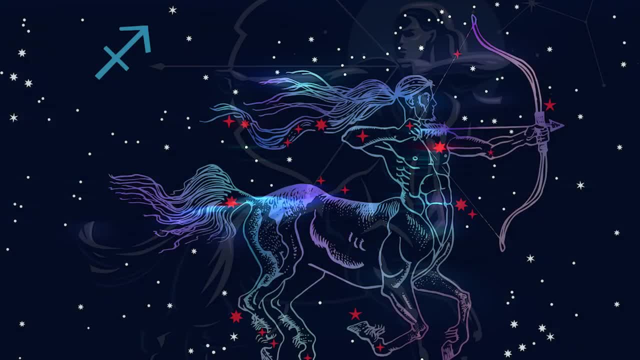 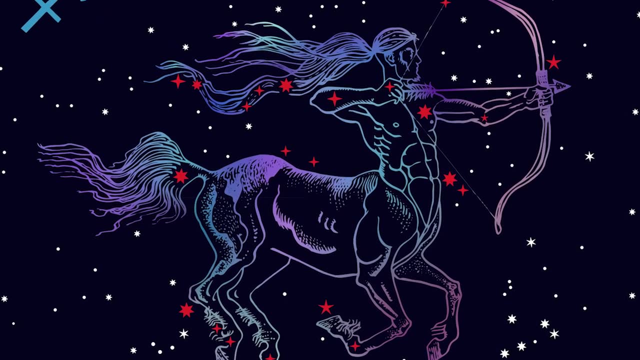 history in Greek mythology. Yet, curiously, there are two depictions of the centaur. One of them state him as just a regular centaur, while the others state that it's an archer and possibly the father of archery. One of the reasons for this is that one of the stars is said to be the tip of the arrow. 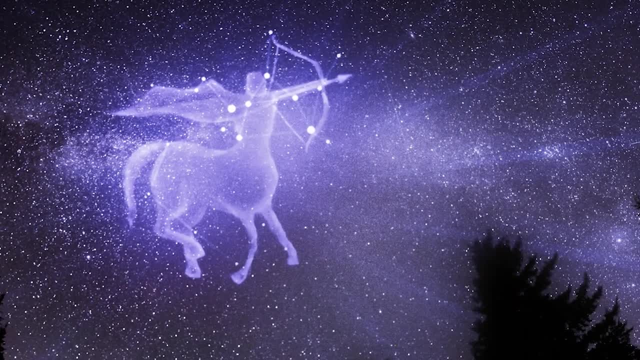 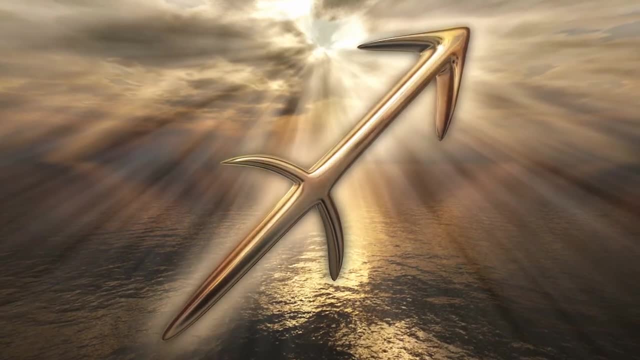 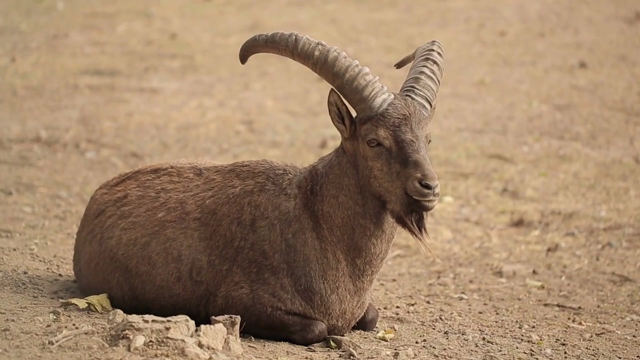 it's drawing. Regardless, the creature is a proud member of the zodiac and centaurs continue to be in all sorts of media because of their impressive stature, and some are even shown to be archers 3. Capricorn: To be clear, this is a goat, not a ram like. 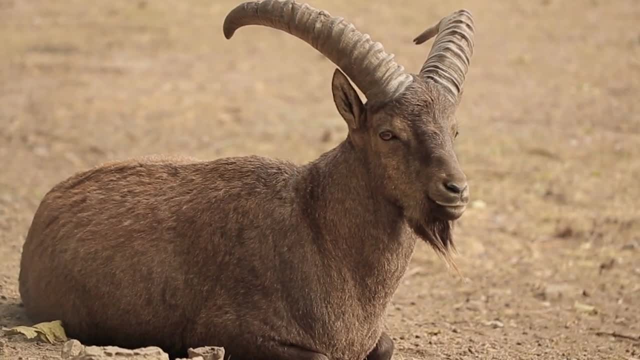 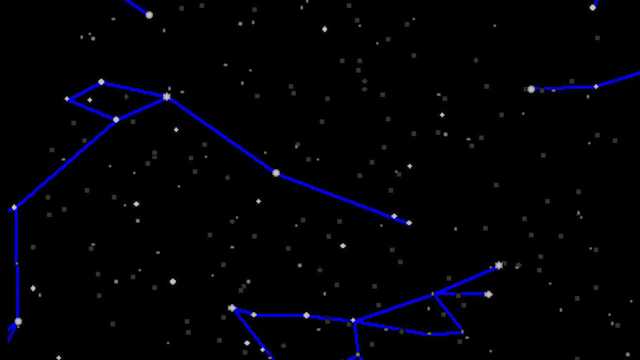 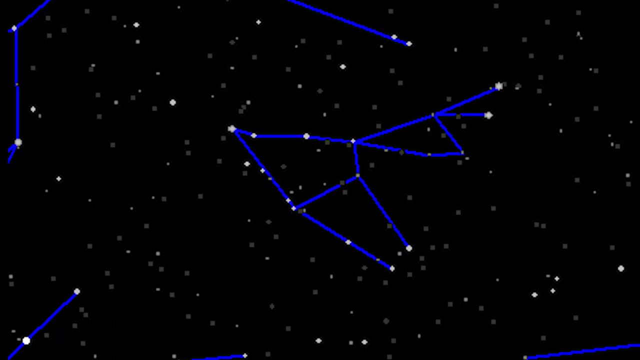 Aries. Thus, this is an entirely different constellation. Ok, We good. Good, I'll move on then. Capricorn is passed by the Sun at January 19th till February 15th and is made up of stars such as Deneb El-Gedi, Dabi Sakuna, Gedi Nashira and more. 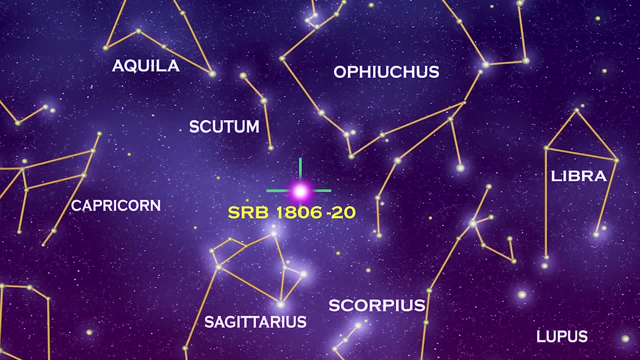 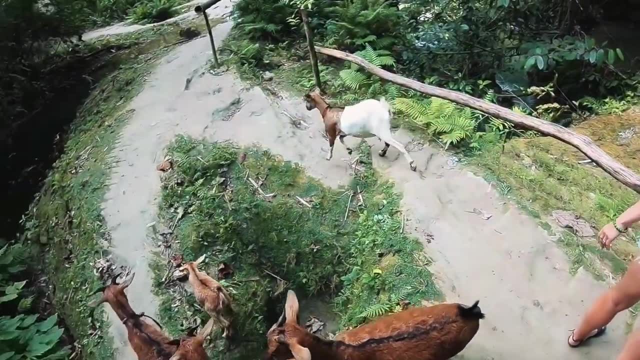 It's one of the constellations that is relatively close to Earth, as one of its stars is only 39 light years away. That's closer than you think. Like many myths, there are several interpretations to this goat, but one stands out. Mainly in Greek mythology. it's said that Capricorn was named Amalthea, and it was her who saved Zeus from being eaten by his father, Cronus, who tried to prevent the prophecy of his death by the hands of Zeus. Her doing so set events in motion to let Zeus kill his father, save his siblings and rule over the world. She was later put into the stars as a tribute. 4. Aquarius: Known as the Water Carrier, Aquarius is a constellation that has gotten some interesting. 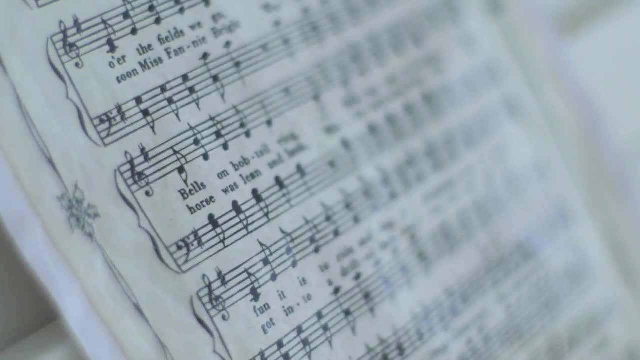 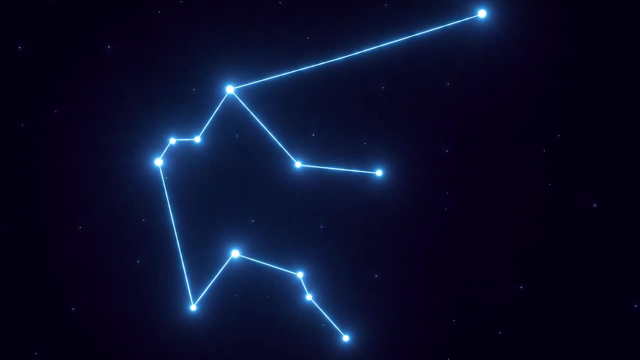 popularity over the years, including a song via Age of Aquarius. It's passed by the Sun on February 16th till March 11th and is made up of stars like Zandeslud, Skat, Albali and more. The closest star in the constellation is about 760 light years from Earth right now. Despite being known as the Water Carrier, Aquarius is not always identifiable. In fact, the first interpretation of the character wasn't a being at all, but a vase.